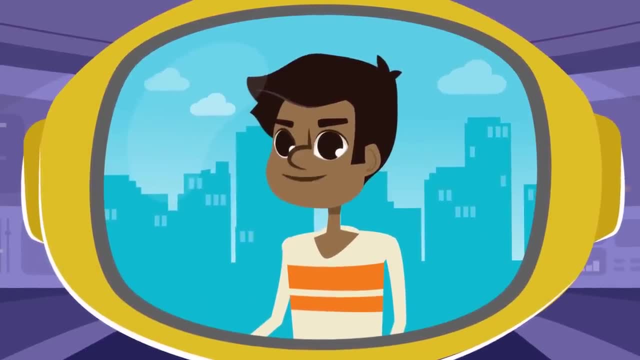 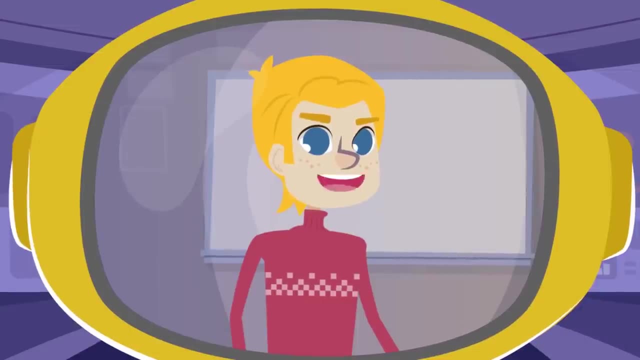 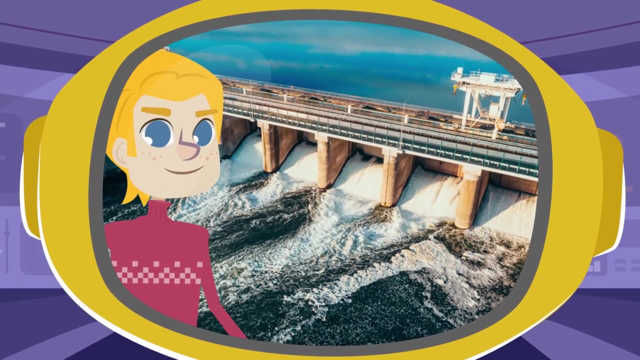 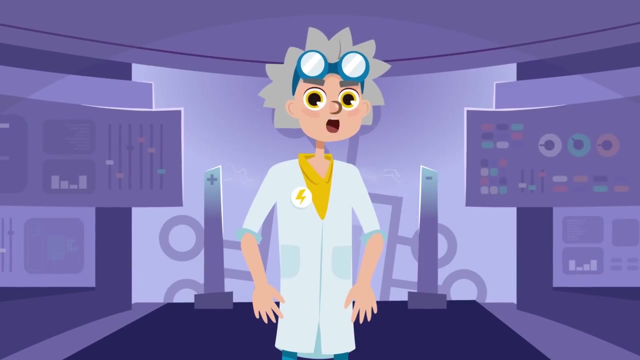 Not only that: with electricity we can power trains and amusement park rides. My teacher told us that we can create electricity by using the energy from natural resources such as water, oil or even the sun. Thanks, guys. I think we learned a lot from our friends. 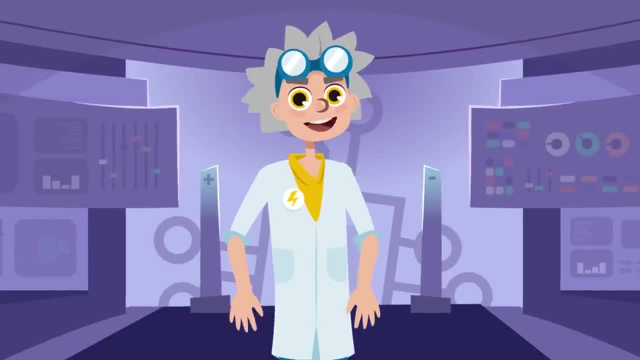 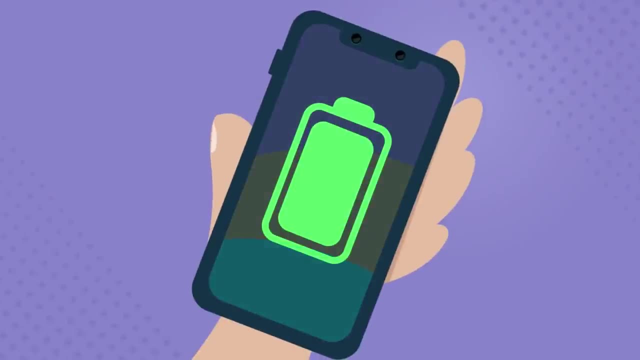 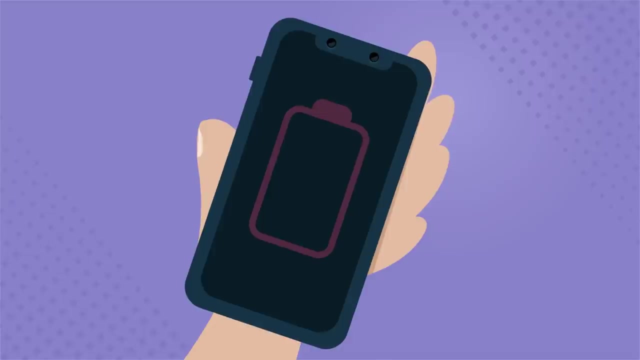 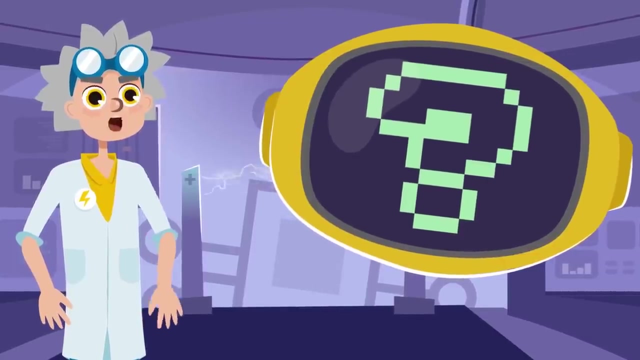 As we saw, electricity is a type of energy we use to turn on lights or power our electronic devices. Electricity has become so important in our lives that we can't imagine living without it. As our last friend said friend said, electricity can be produced in many different ways. let's find out we. 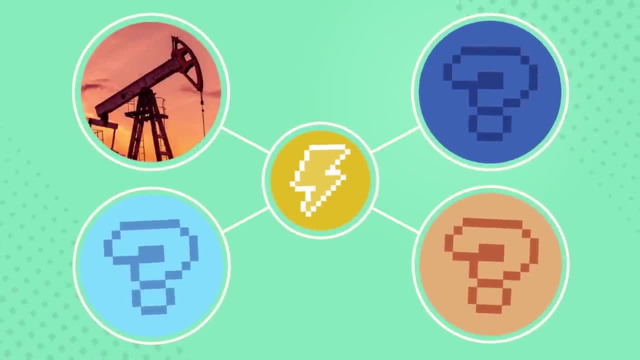 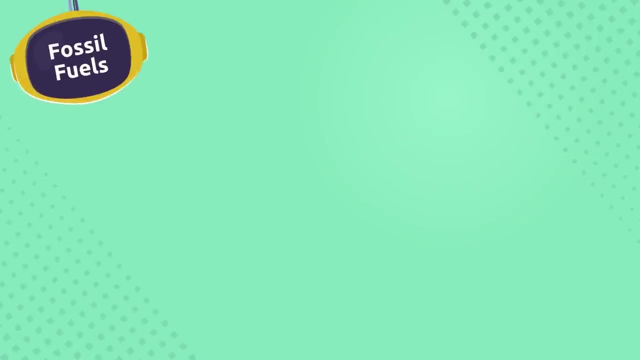 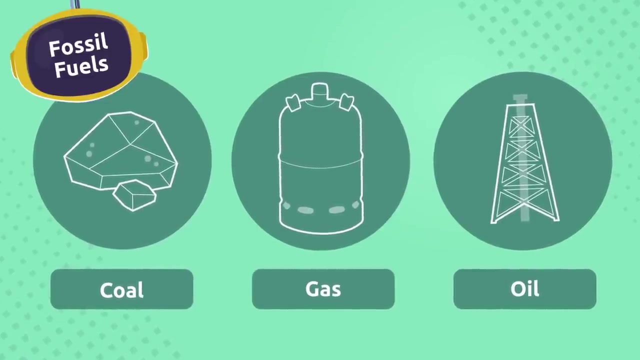 can use energy from natural resources like fossil fuels, wind, water and the Sun to create electricity. let's take a look. fossil fuels such as coal, gas and oil are natural resources found beneath the Earth's surface. we burn these fossil fuels at power plants to boil large amounts of water. this produces steam. 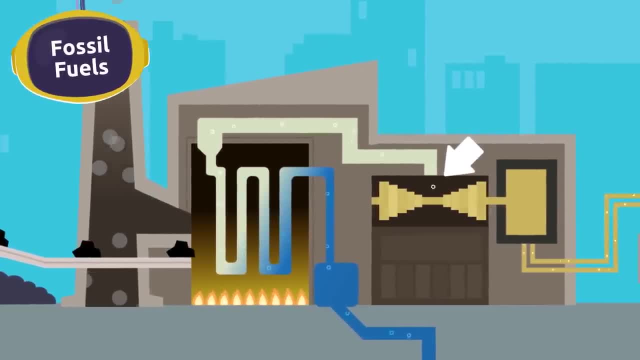 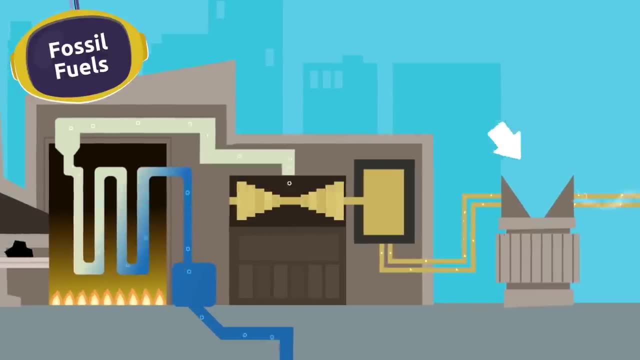 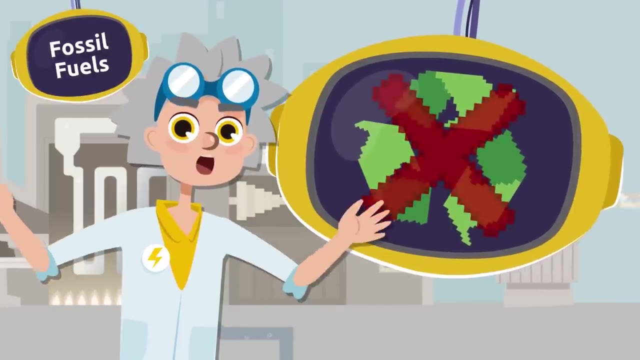 that is powerful enough to turn a large turbine, which basically looks like a big egg beater. when the turbines turn, they activate a generator that produces electricity. but we have to be careful because producing electricity with fossil fuels is harmful to the environment. another way we can get 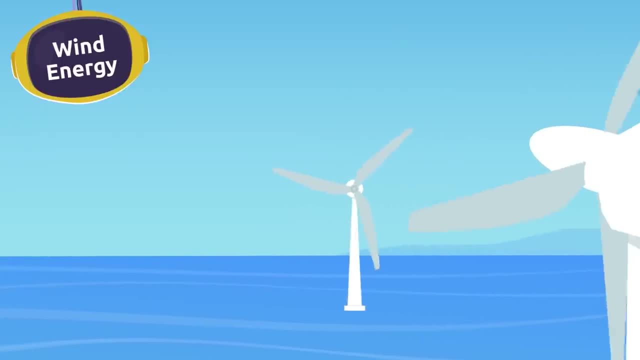 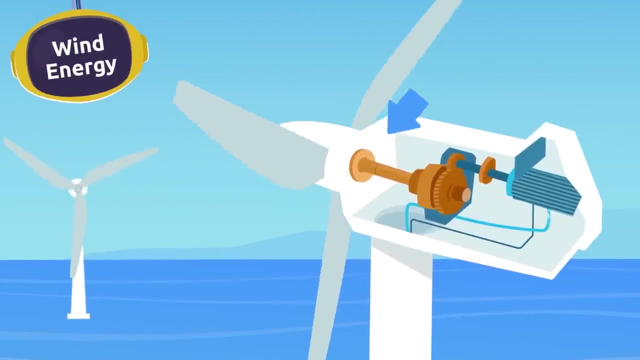 electricity is by using the fossil fuels that are produced in the environment, in other words, wind energy. have you ever seen wind turbines? when the wind blows and pushes the blades of the wind turbines in a circular motion, it also turns a shaft, which activates the generator producing electricity. we can. 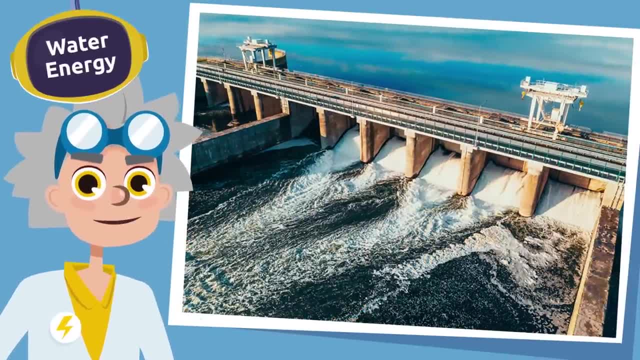 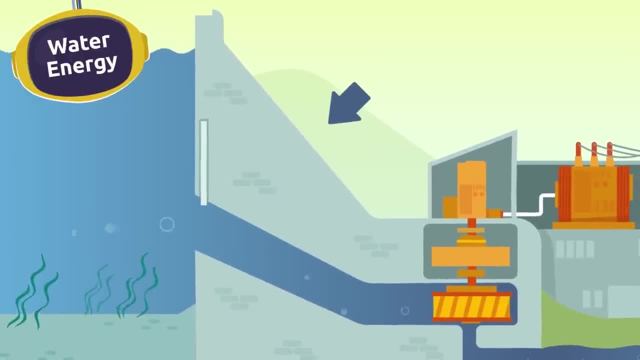 also get energy from the force of the water. maybe you have seen a dam. it is a big wall of fossil fuels. we can also get energy from the force of the water. maybe you have seen a dam. it is a big wall of fossil fuels built to collect large amounts of water. the water is pushed through pipes which